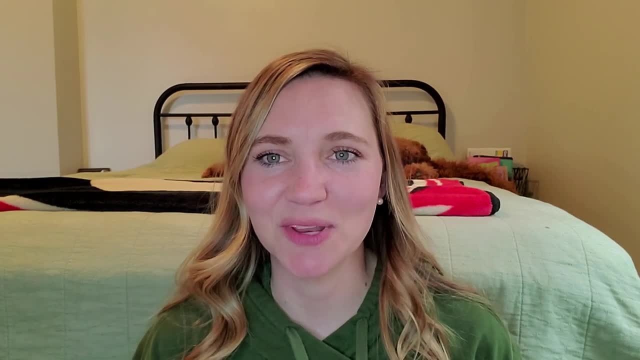 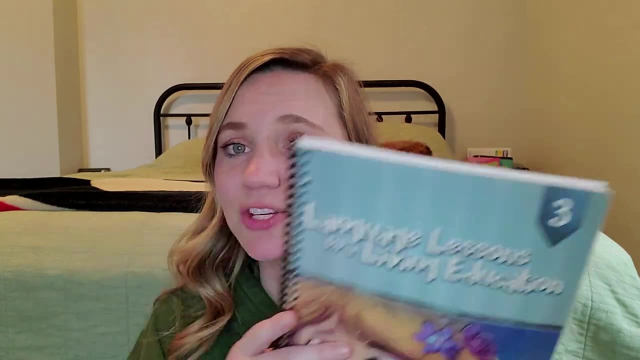 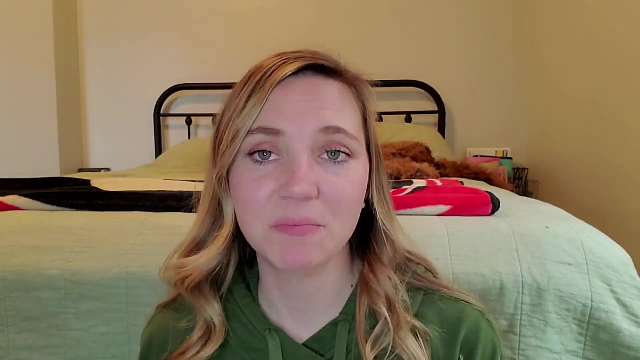 down in the description box below. We would love for you to join our community here. So, as I said in the intro, I am going to be talking about language lessons for a living education three and language lessons for a living education two. We have just finished this up back in a. 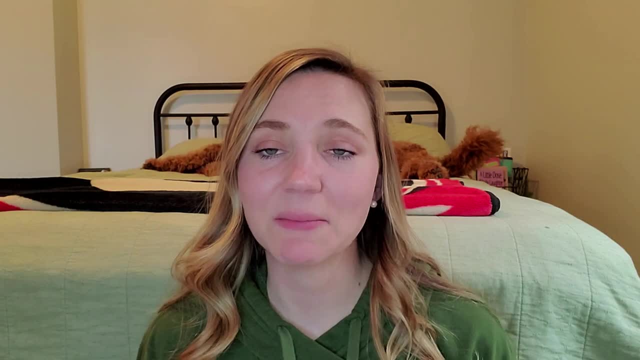 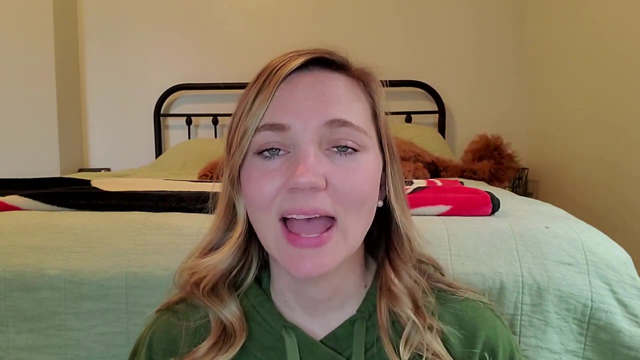 December. I'm going to be talking about language lessons for a living, education, three and language, and so we are moving on to something else. I'm going to talk about what we loved about it, what we didn't love and why, ultimately, we are moving on from that. I know this is going to come up because 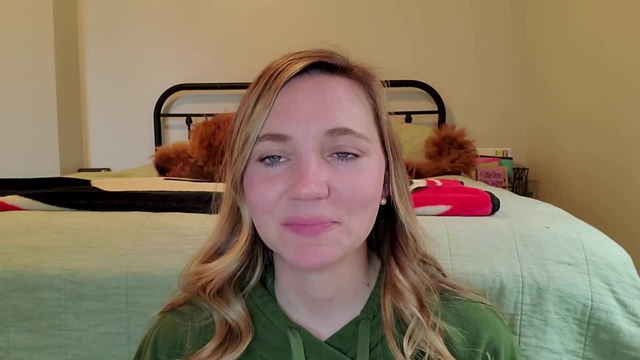 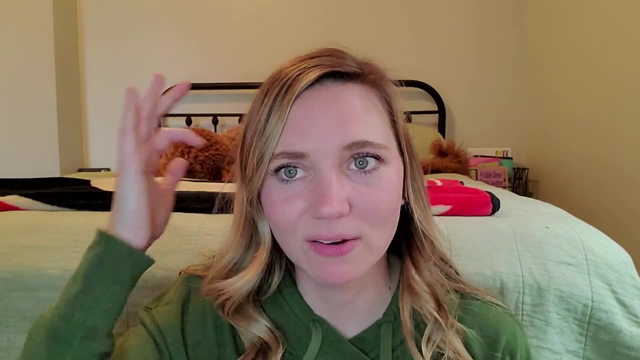 he's back there making a ton of noise, but my golden doodle, Noah, is back on the bed. I just realized I have like two videos in of filming and he's back there. He wasn't moving earlier, but he's moving now. Everybody comments on the fact that he's back there. He is never more than five feet. 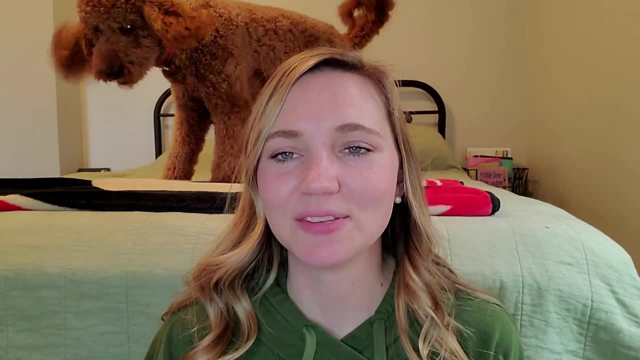 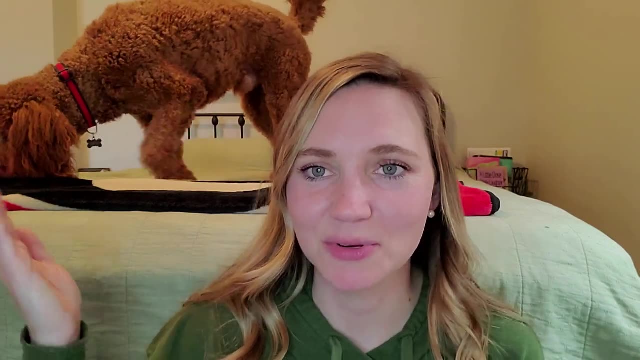 away from me, So you see him in the background of a lot of my videos. Thanks, bud. So anyway, that is Noah. That's the Noah the farm doodle. At least he's not over here in between me and the camera. He usually 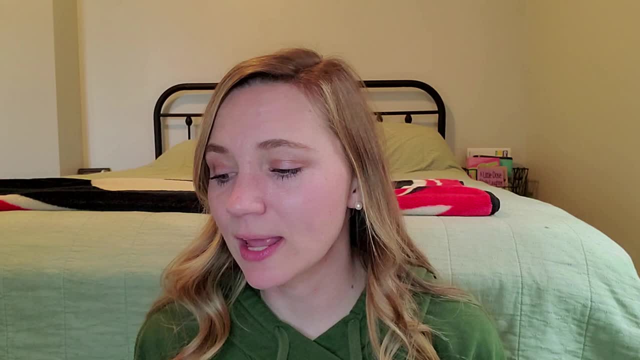 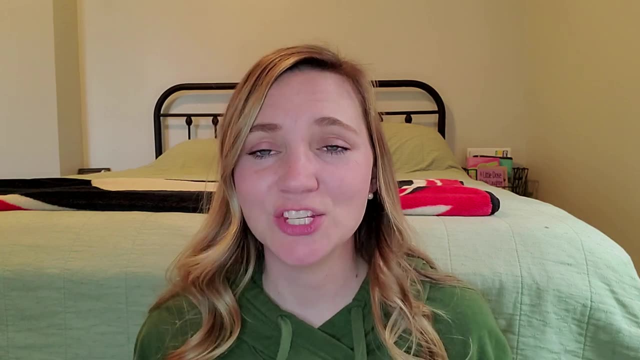 that's. he likes to do that too. So anyway, let's get started. So I am just going to kind of briefly walk you through it. I think I have a flip through of this up on my, on my channel. If I do, I will. 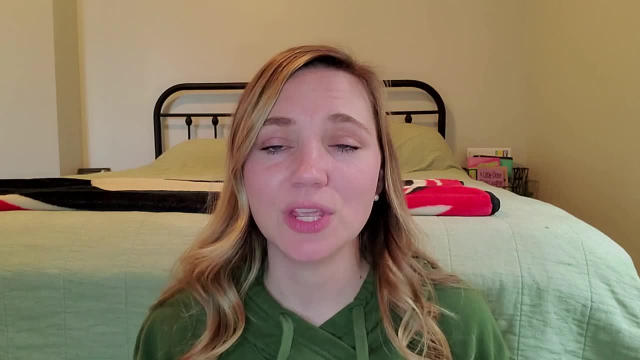 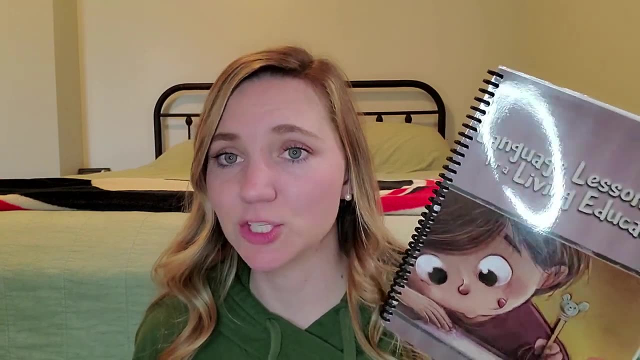 put that up here in the iCards and link it down below so that you can see that. I think it's just a level two, Maybe three, two, I can't remember. It's been a while since I've done it. Like I said, we started. 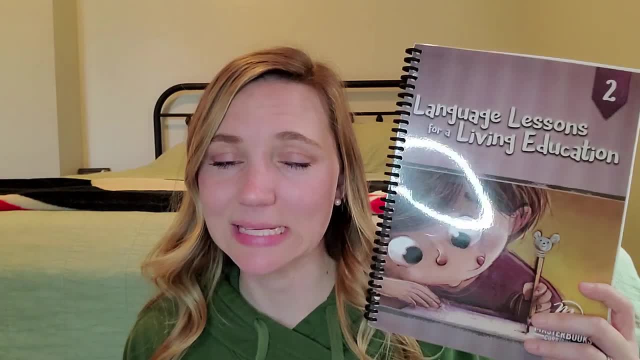 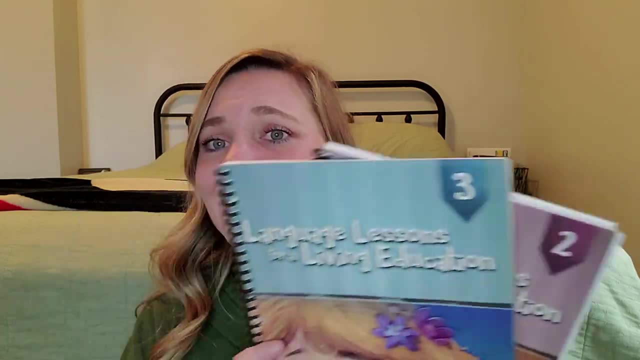 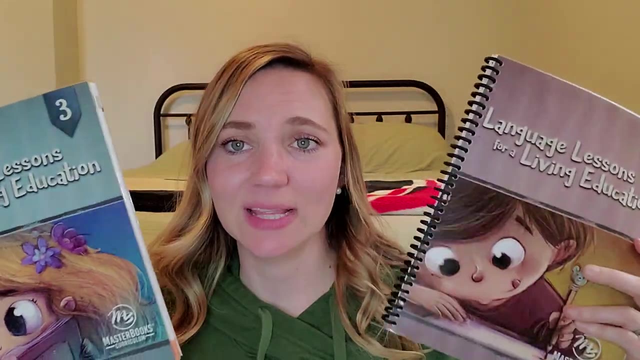 this in January of 2021.. It is now January of 2022.. We've gone all the way through this curriculum and you will notice that it looks differently than when you buy it. What I did is I took things that were very like that should have been in a teacher's manual. I took it out and I 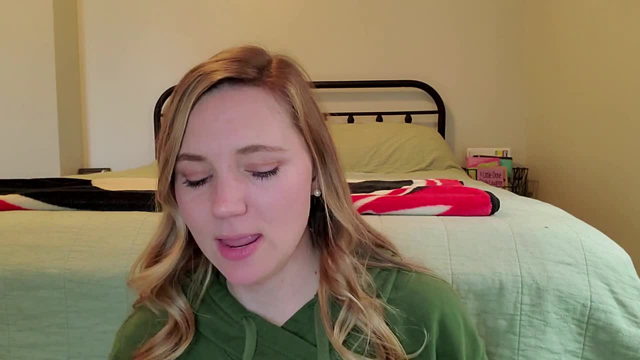 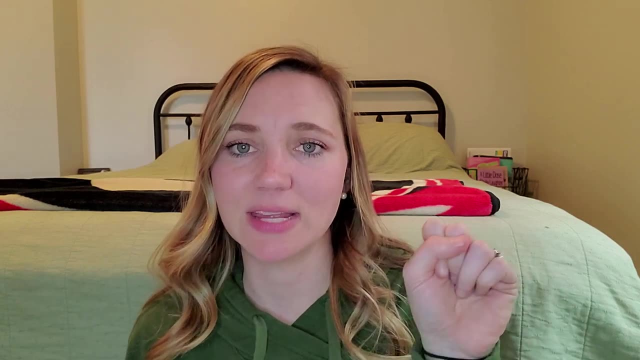 bound it so that it would be easy access for me. I put everything that the kids needed into a binder so that they could open it. I have a kid that's left handed, And so the when you open a book, the like heel of the book drives her nuts. 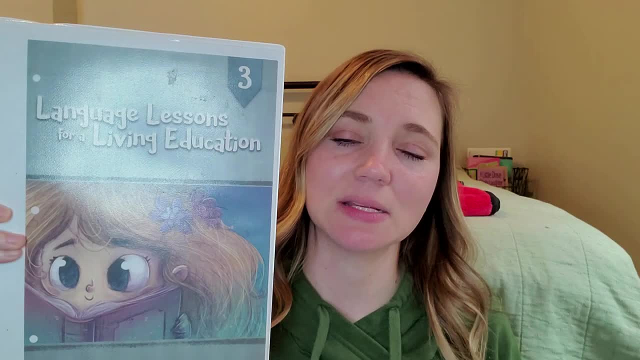 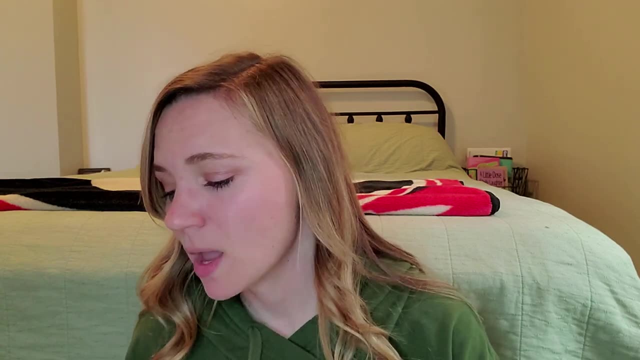 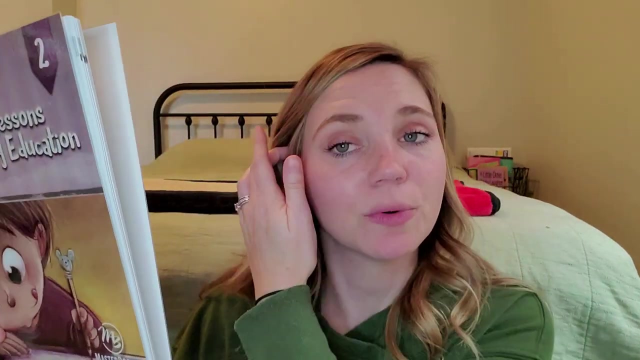 So a lot of times taking things out of workbooks and putting them into binders is very helpful for her. So I did that with all of my master book stuff and it was. it was very helpful, So I'm trying to figure out where to start. Okay, so language lessons for a living education too. 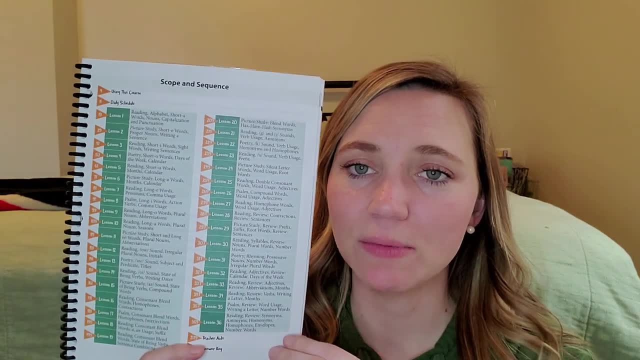 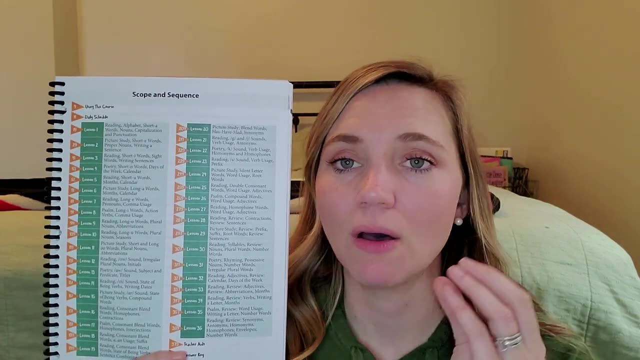 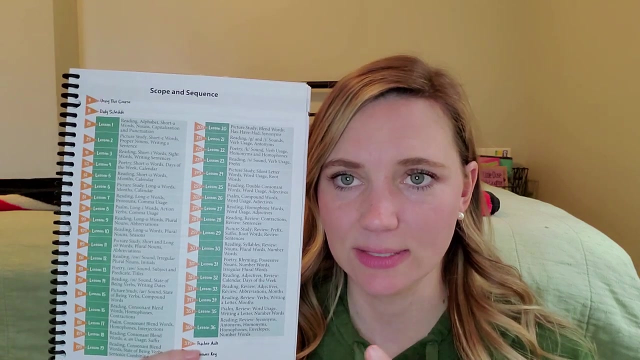 What I liked about this is the fact that everything for language arts was included into one book And in a season of life where we needed it to very open and go. we didn't need a lot of things, a lot of extra things, a lot of flashcards, a lot of manipulatives and all the things. 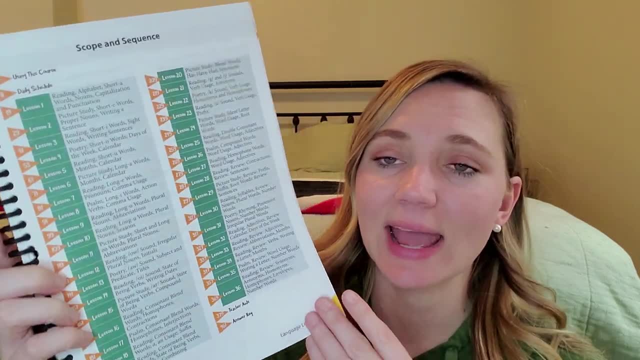 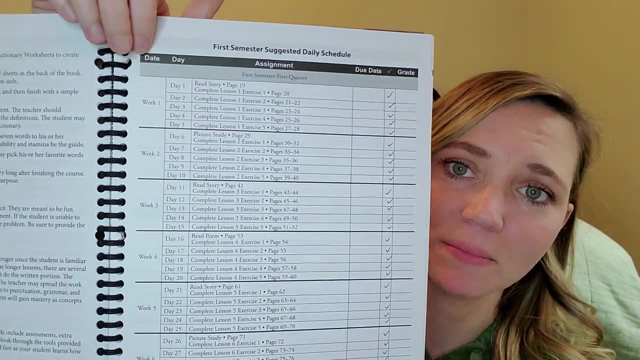 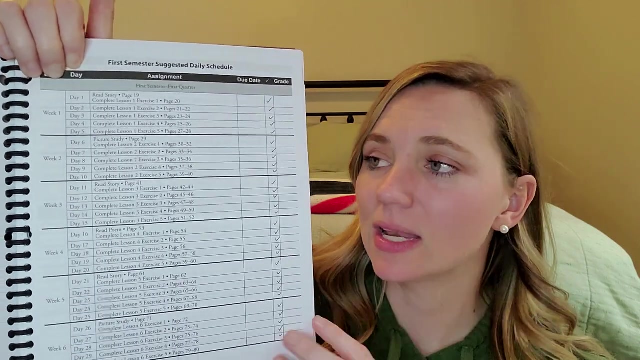 This curriculum was very helpful for us. It had everything that we needed in there. They even broke it down into a schedule of the weeks and how you broke up. the lessons were in here and you could check it off and agree and to a grade. It was all there. 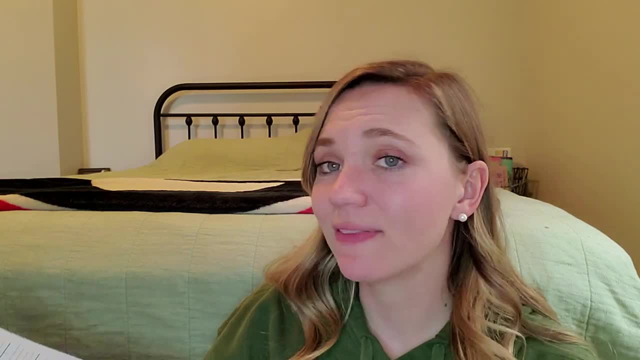 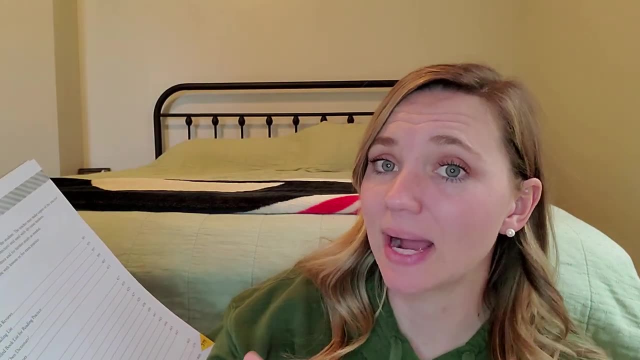 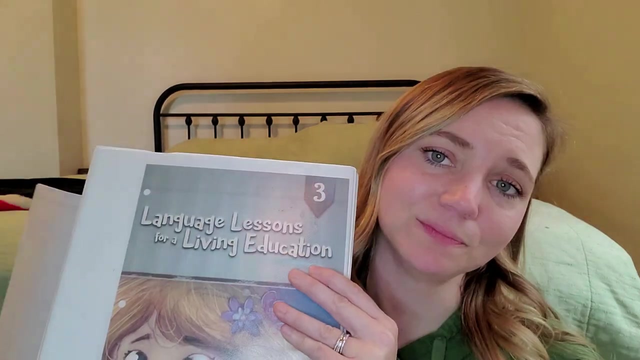 ready for you to use. So I thought that part was very, very helpful. And then you have your teacher aids. I think this is in the back of the book, So this is where, like it all, where I took it apart. So then you have your lessons and then you have what your teacher aids in the back. 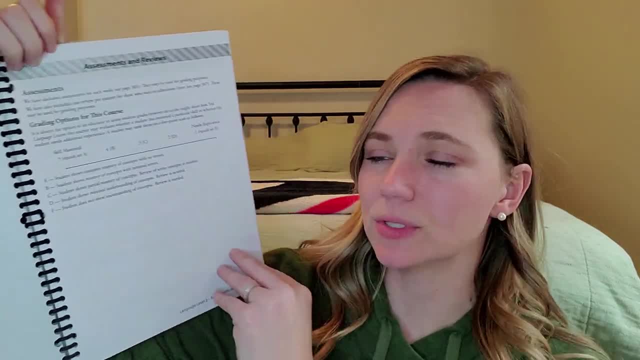 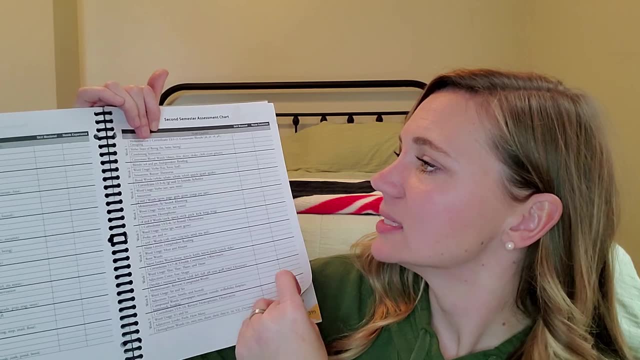 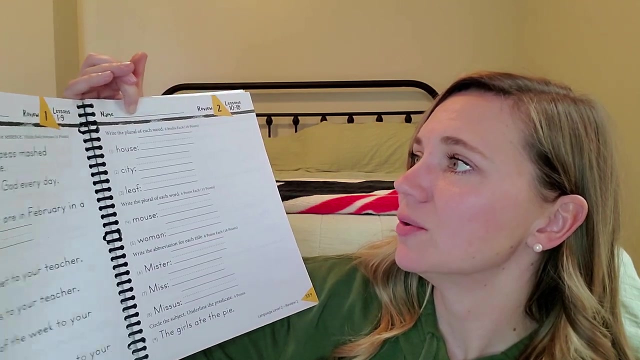 so and you have your assessment and reviews. You have- I'm trying to hold this up- I probably should have done this- laying down Assessment chart where you can, any assessments that you did. you can write it down and just see what they knew You. 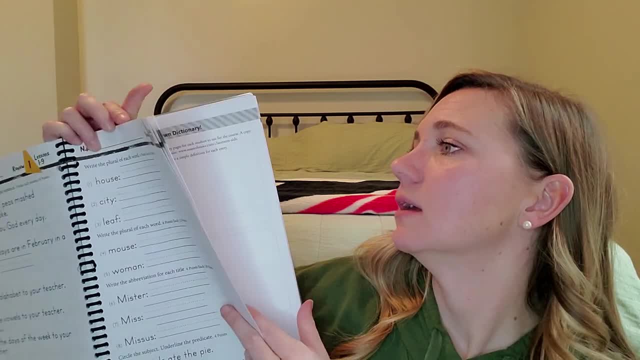 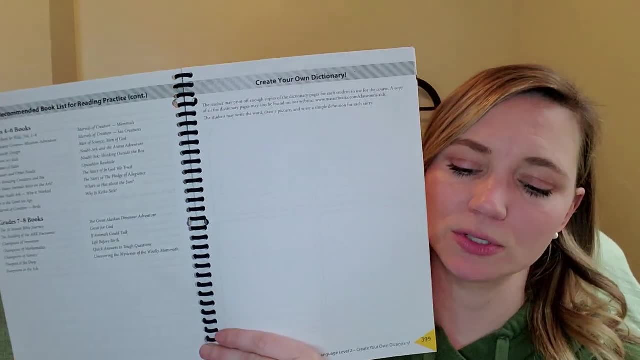 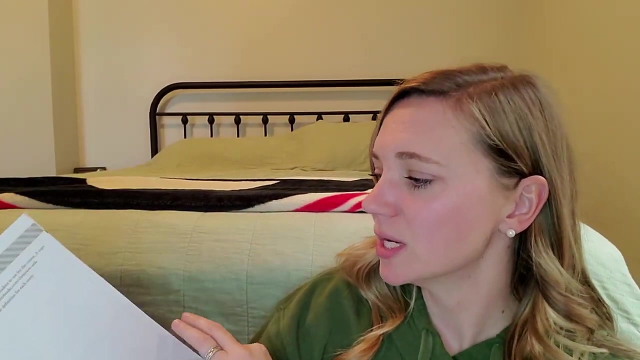 have review lessons if you wanted to do that. You have book lists from Masterbooks, So the book, their book list, is only going to cover what Masterbooks- sorry, what Masterbooks- sells. This is not anything outside of the Masterbooks publishing company. 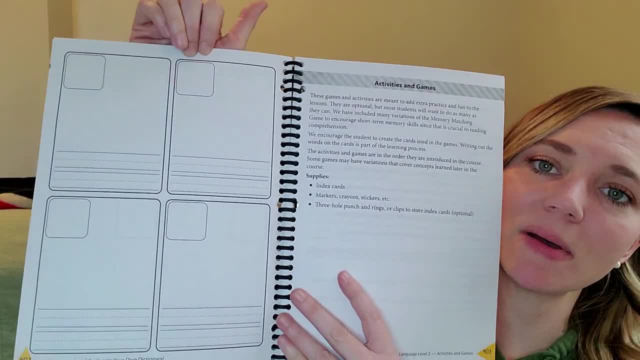 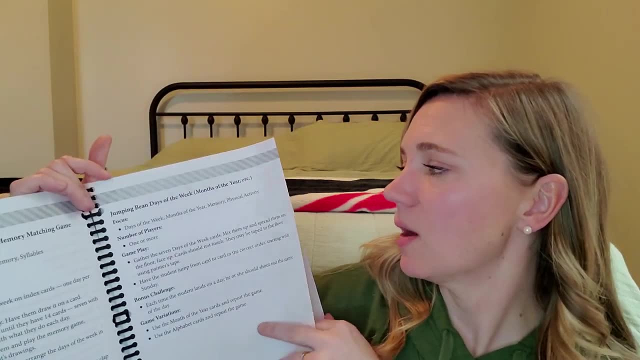 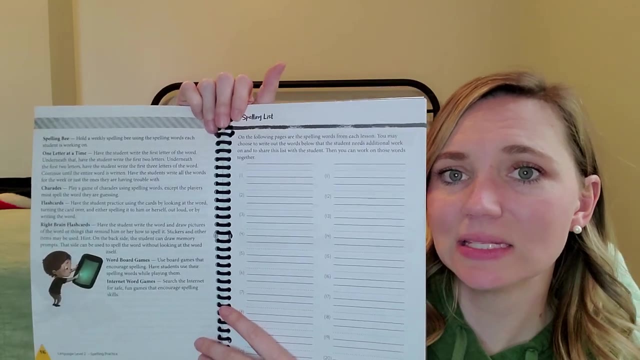 You have pages for making your own dictionary. in the back You have activity and game suggestions that you could do to help with learning different concepts. You have spelling list that you could make copies of, and they do give you full rights to make copies of anything that you need to. 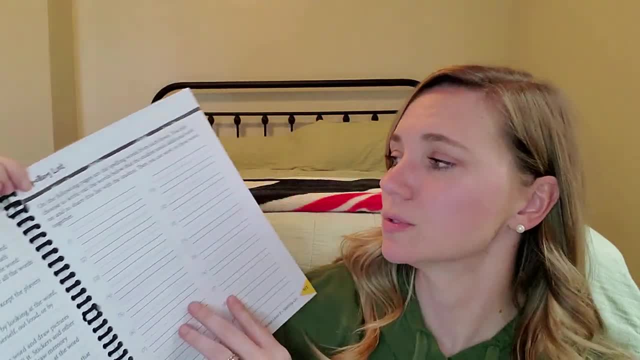 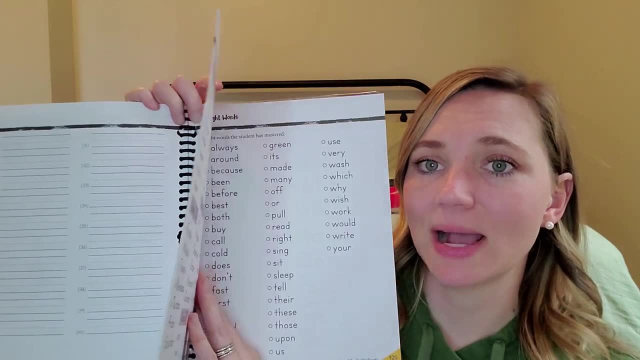 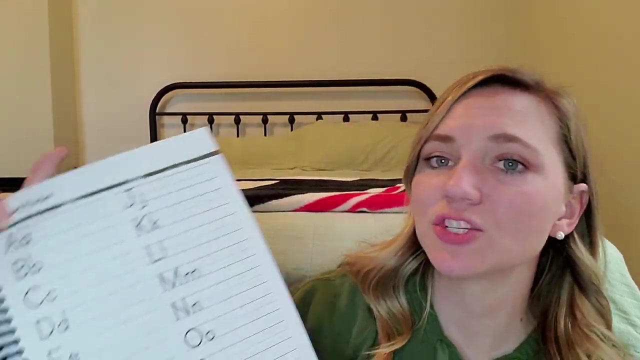 as long as it's used within your family, your household, So it's not like you could pass this to like a co-op or something. All the spelling lists for the weeks are in the back of the book or you could get to that. You have sight words in here and then you have extra practice for. 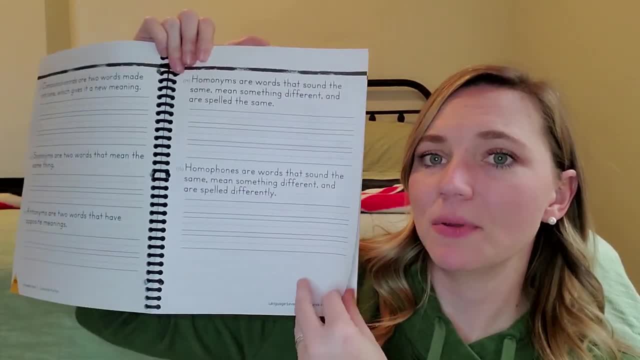 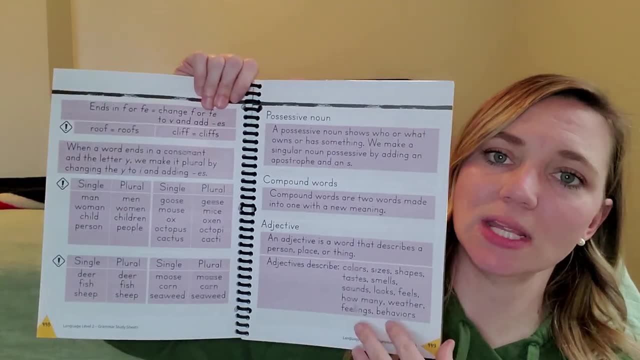 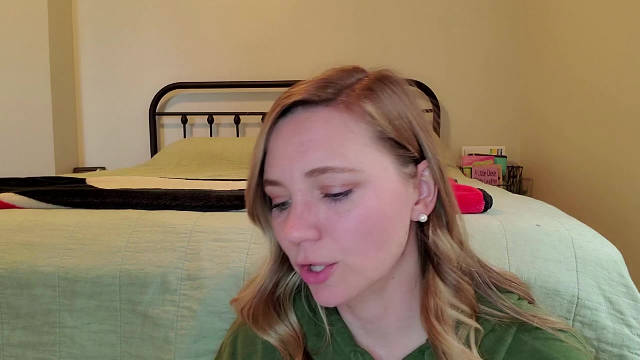 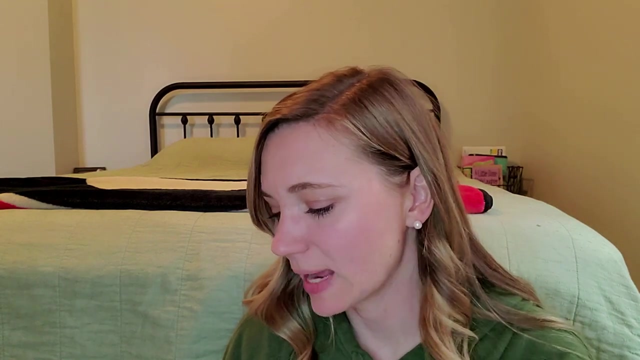 like writing handwriting. um copy work is in here And then you have these study pages in the back. It has everything that you need to know about as far as, like contractions, singular, singular plural subject predicate commas. you know anything that you would need to come back. 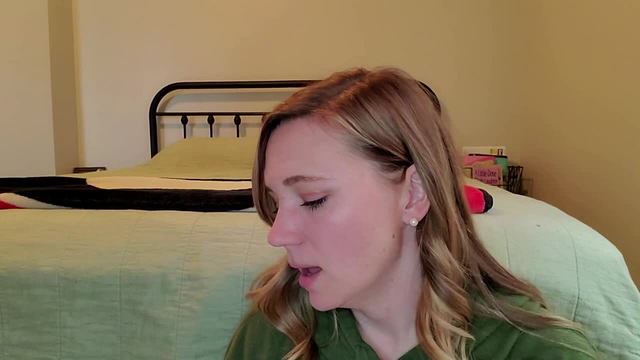 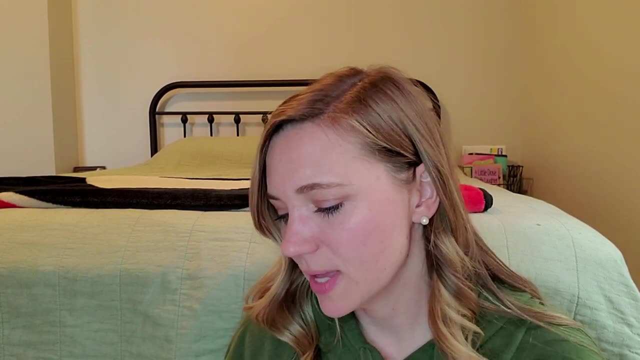 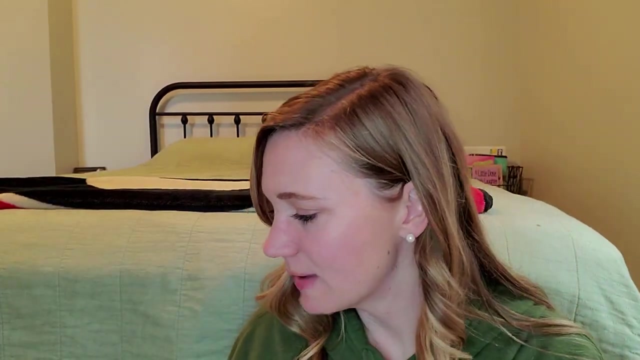 and reference, reference. homophones, homonyms, um, different verbs, tenses and initials, titles, suffixes, root words, contractions. All of that stuff is back here in the back in these study pages. And then you do have answer. You have an answer key in the very back of the book. So everything is. 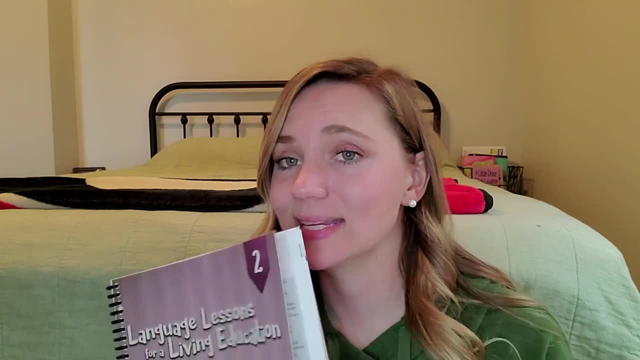 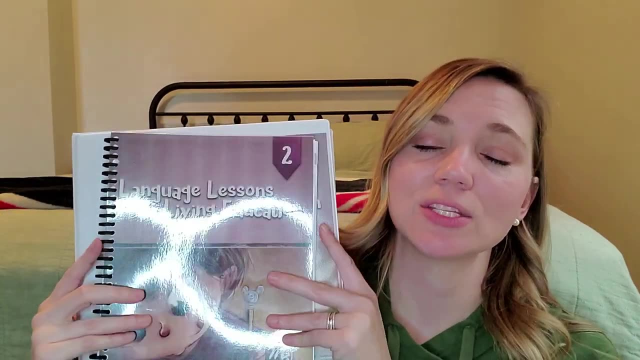 here. The one problem I had with this, and one reason why I did not like it, is because it was all in one book One. it all came in one bound book So you don't have like its own teacher's manual. You, if you're sitting down and doing this with your child, you have to look over their 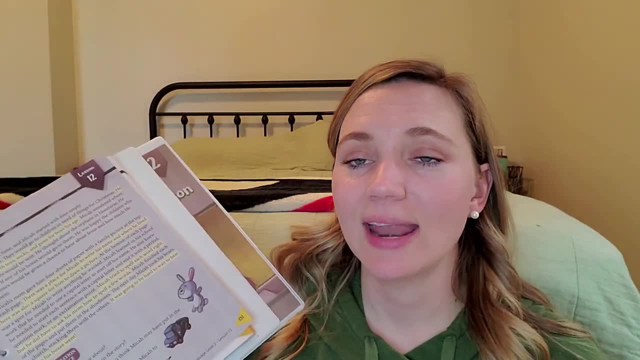 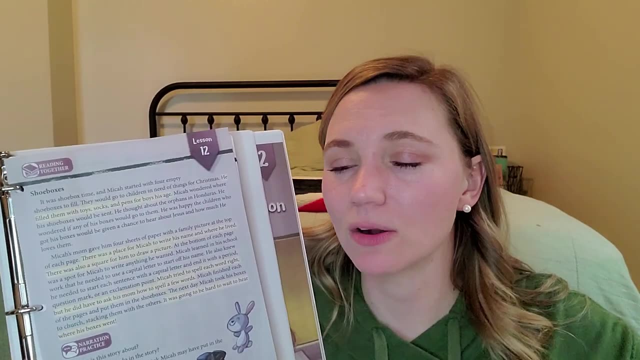 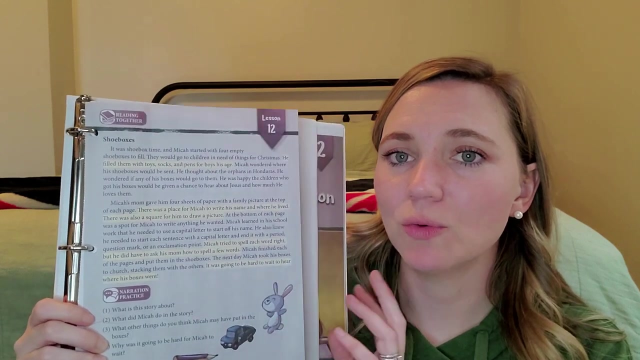 shoulder. And as far as looking at to some of the lessons, and I our starts at lesson 12, because we had a lesson one through 11 last school year And so all of that has already been filed away with last year school work. Um, so the way that this starts off is is every you rotate between having 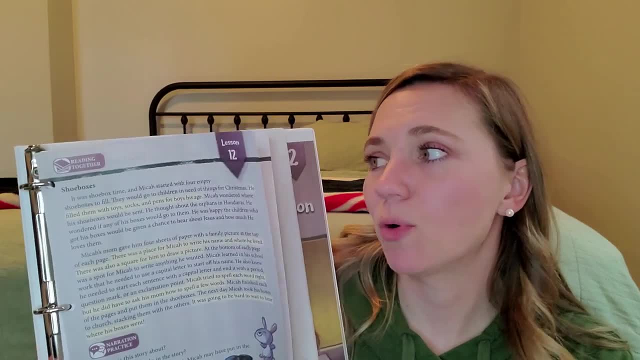 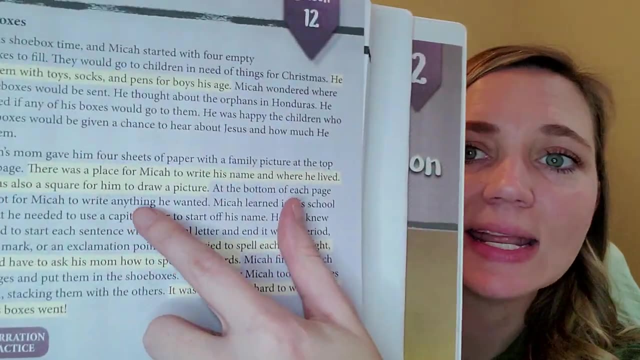 a story and having a picture study or having a point of going over poetry or Psalm or something like this. So on the first page you have a story. The highlighted sections are what your child reads. The rest of it is what you read. 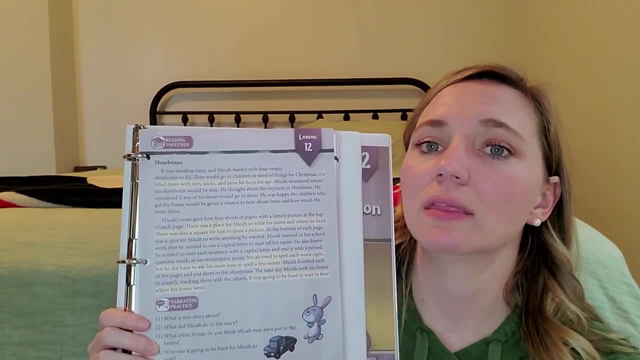 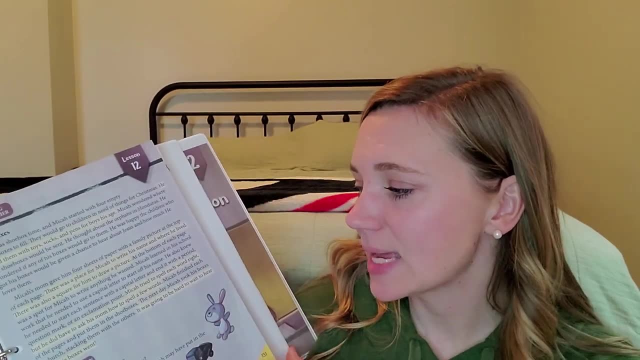 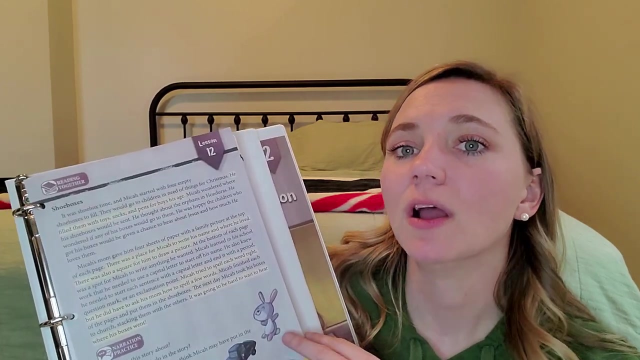 So what you considered your kids reading for the um, for the course, is reading through the story, this story, And the first day of the week it does say to do like 20 minutes of reading time through the rest of like along with your kid as like silent reading or whatever. but there's not. 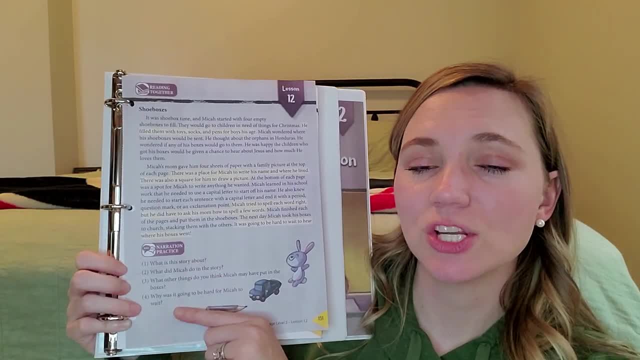 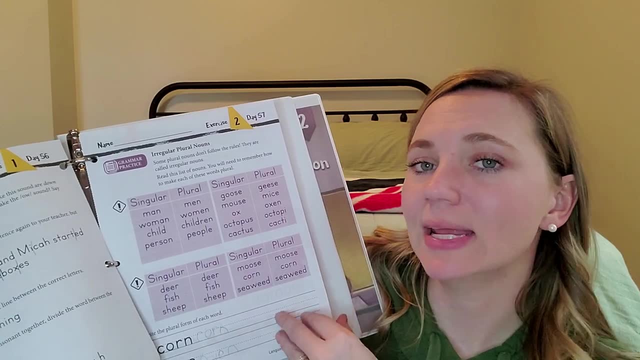 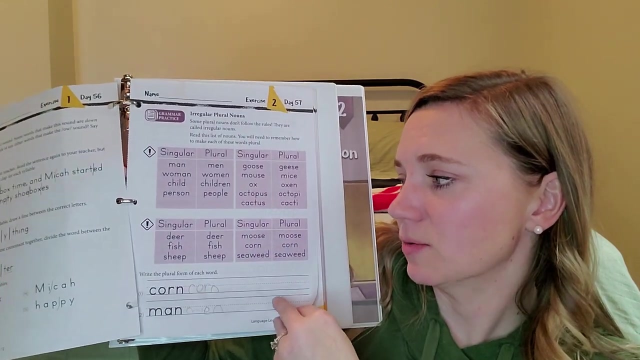 like a comprehension. This, this is it. So you have narration practice where you ask them questions based upon what you talked about. Then you go into grammar writing that they're doing, So this is like your teaching material right here in the book, And then this is their practice, right? 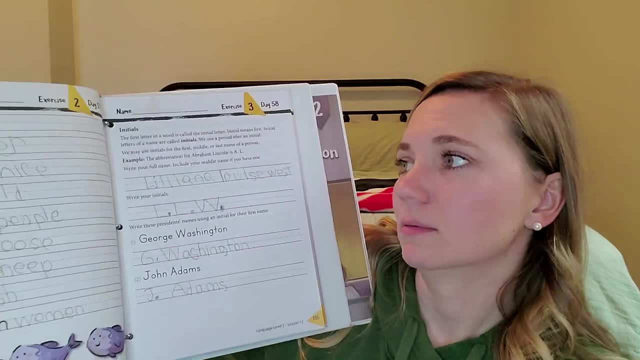 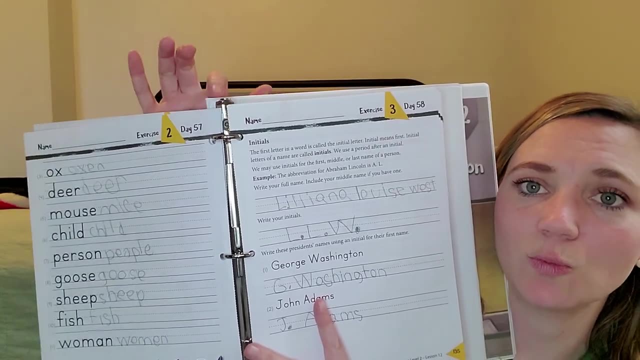 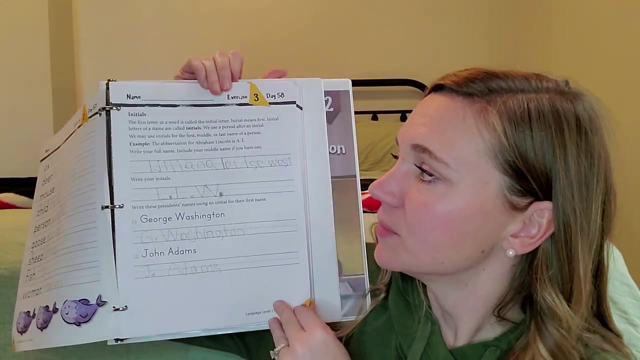 here, right, The plural forms of each noun there. And so this is their practice, and that is exercise to exercise. Every exercise is one day, So that's all they do for one day, And this is all they, and then this is the next day. Um, here's your teacher and material. Then they go over this. 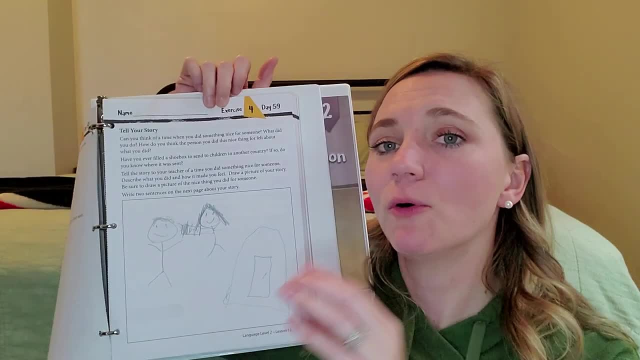 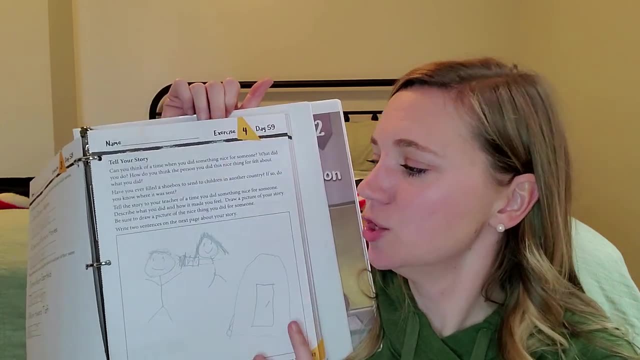 um, and then this is their practice. this On day four, it was always tell a story, and in language arts too. You told a story and then you drew a picture about your story and then you wrote a couple of sentences about your story. 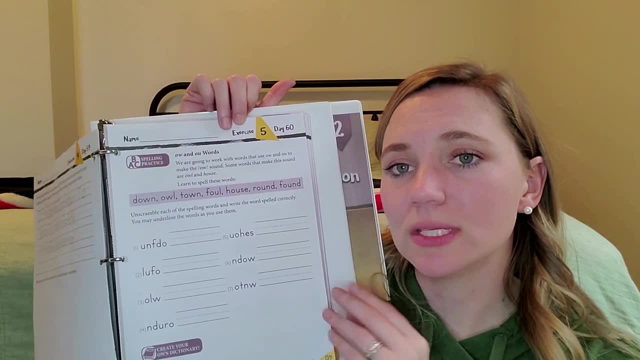 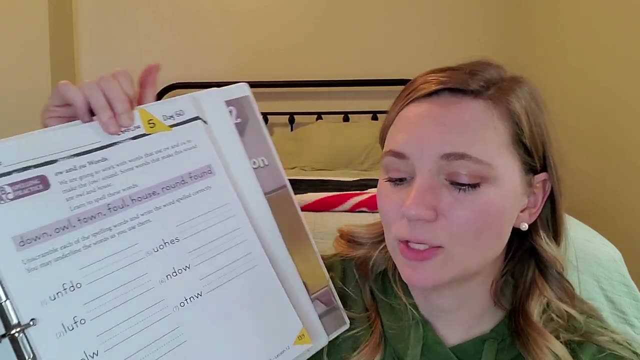 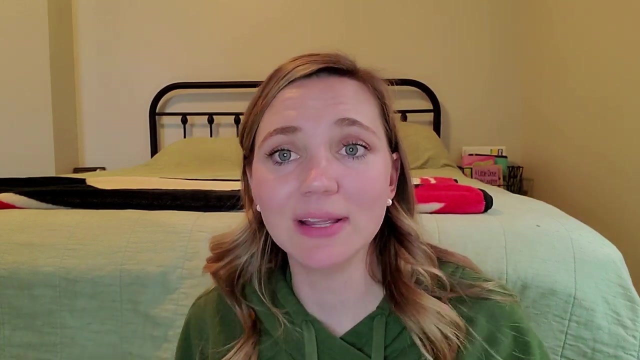 And then day five was spelling and you will notice that none of my kids have their spellings filled out. I did not love the way that master books did spelling, so we did not do the spelling out of this. But one of the pros about this curriculum is everything is in one book. You do. 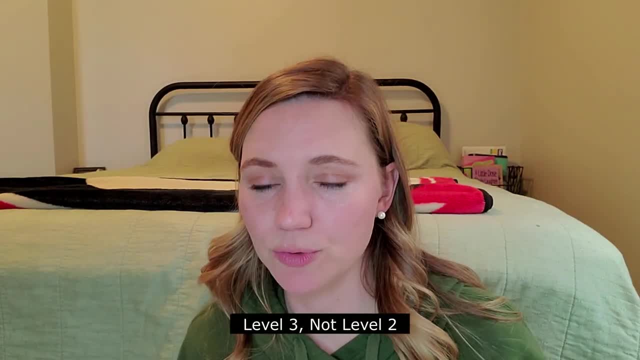 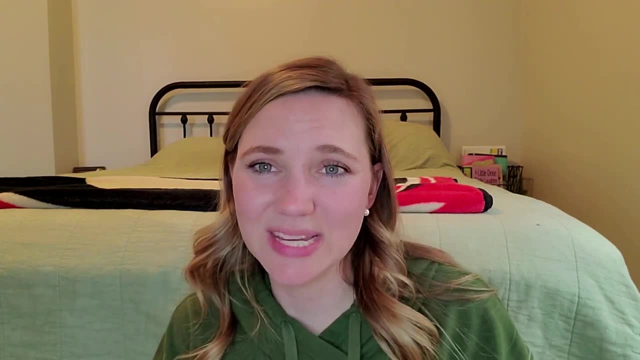 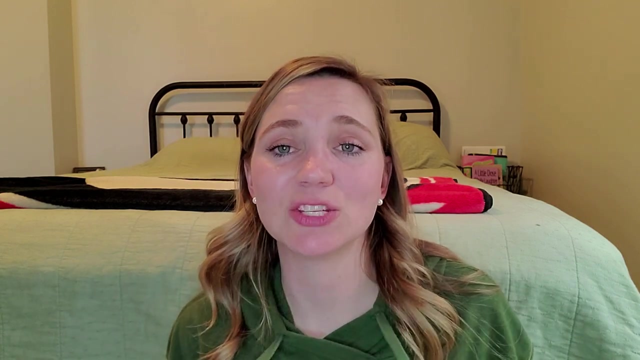 not need to buy extra things, except for when you get to level two. you do need a reader that comes along with it. Things that I did not like about it is the fact there wasn't their own teacher's manual that it was not explaining to me, as the teacher is somebody that struggles with language. 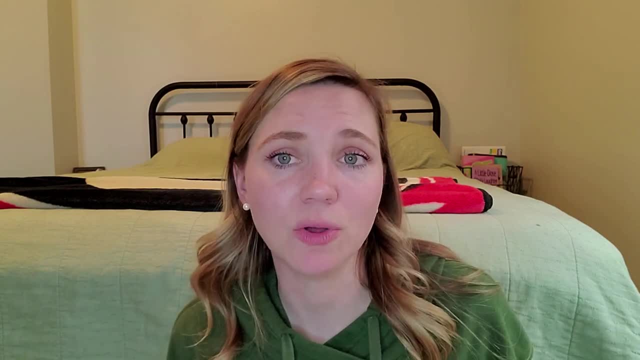 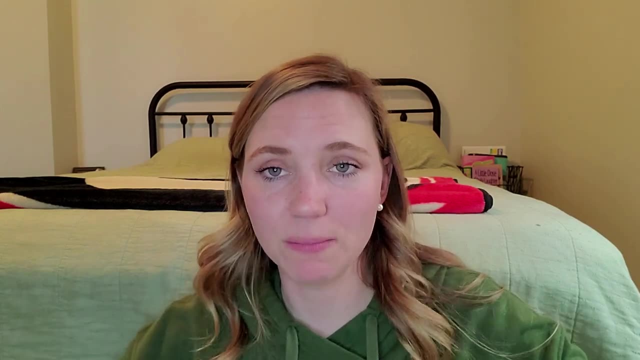 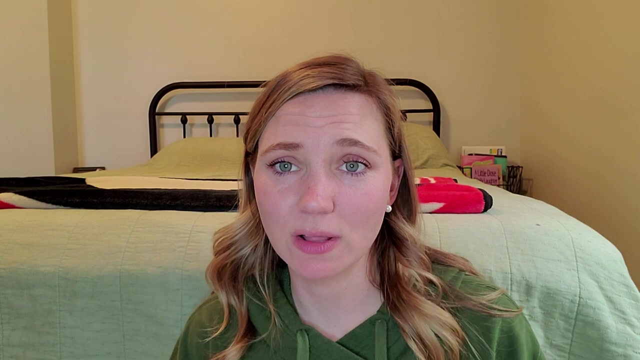 arts stuff on their own. That was not my best subject in school. I felt like I needed more on my end as being a teacher, So that's why we are moving from this curriculum. I felt like if this curriculum is very good for kids that are struggling, 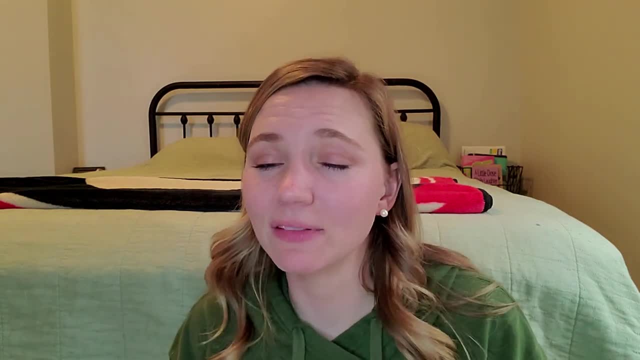 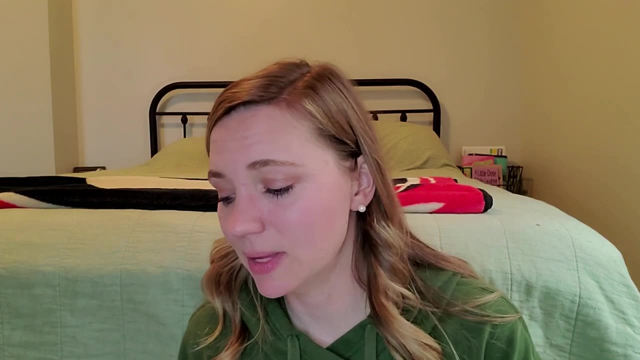 if you had special needs kids. if you are in a season of life where it's very busy and you just need to open a book and you need to go and you're either hand a book to your child and be- if they're fluent readers- and just be like here, do this. 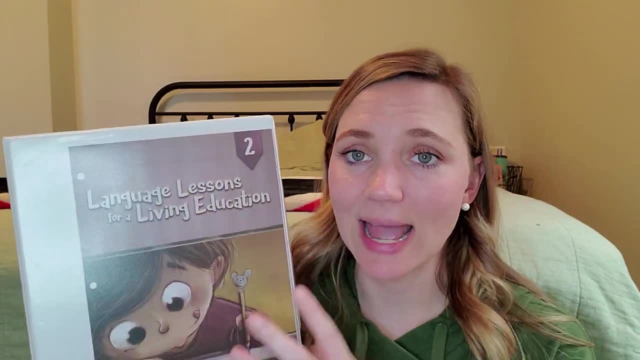 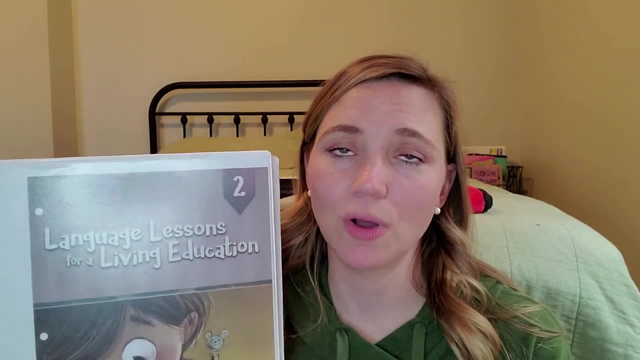 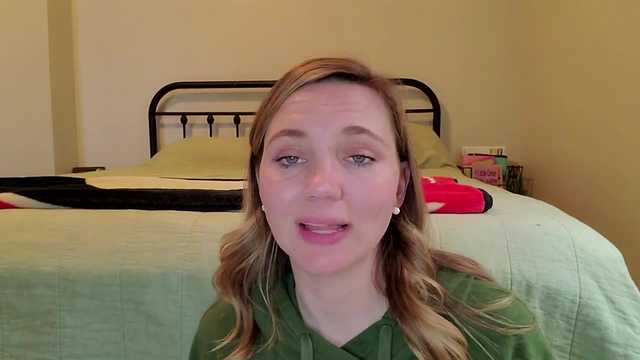 Level and these are leveled. These are not graded like as grade. So this is level two, which, on my opinion, is not a grade two on grade two level. So it's not per like a grade level. There's just a lot of things. I felt like we're missing out of this, that I think it's because 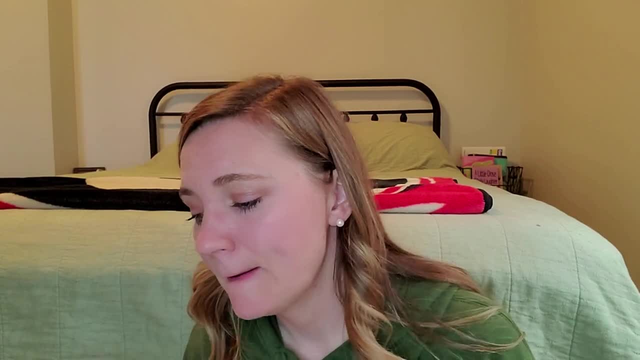 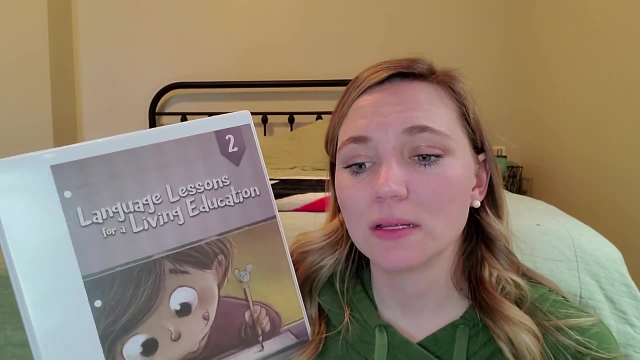 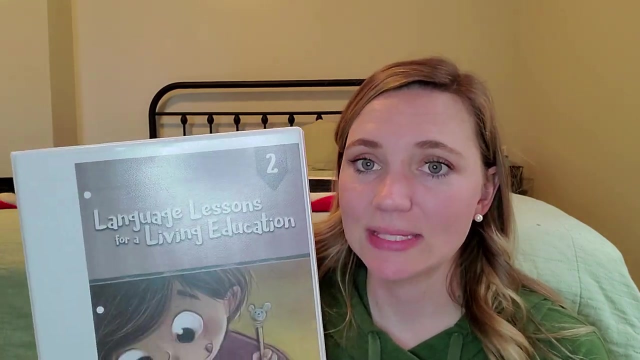 of its approach. Its approach is Charlotte Mason, And not that there's anything wrong with that, but I have just- I have just found that I want things to be when it comes to language, arts and to math. I don't want it to be language to be Charlotte Mason, I want it to be more traditional. So I felt like that was. 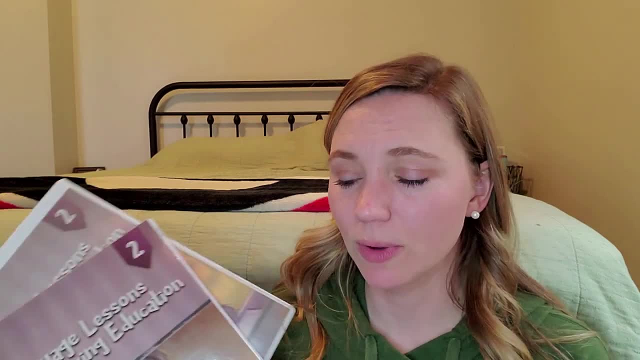 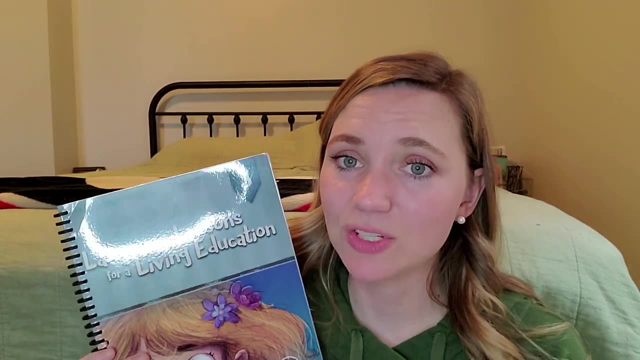 kind of what our hang up was on this. So I'm going to show you really quickly through level three. It's set up pretty much the same. It goes through the same material, just goes a teeny bit deeper. So that's the only difference. 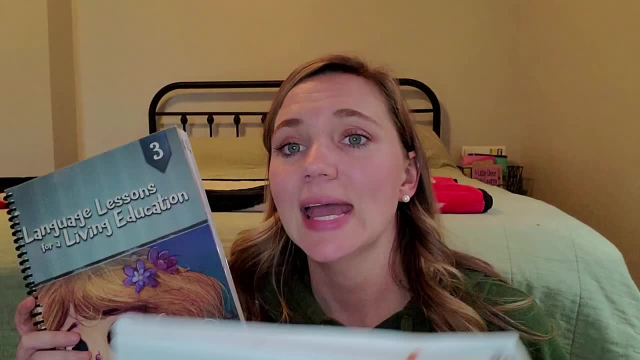 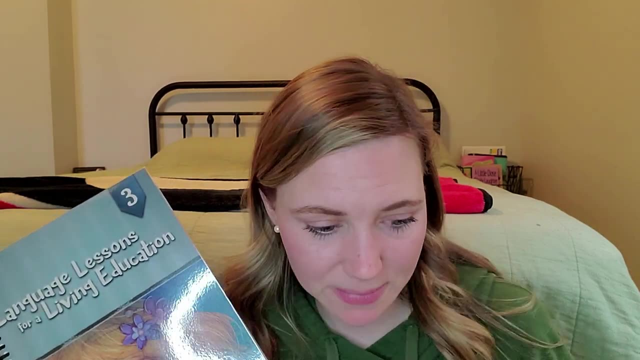 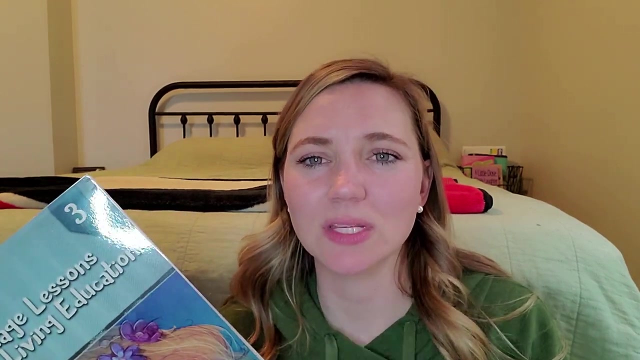 Between level three and level level two is level three goes a little bit deeper, And I also had level four to look through too, And it goes through the same exact material, just a little bit deeper. You did a little bit more with it And I just felt like that wasn't enough. So not again, not that any. 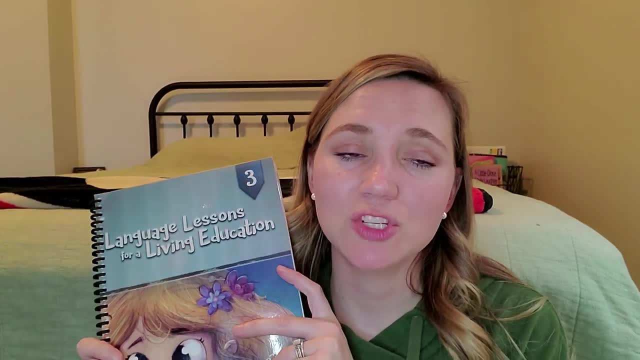 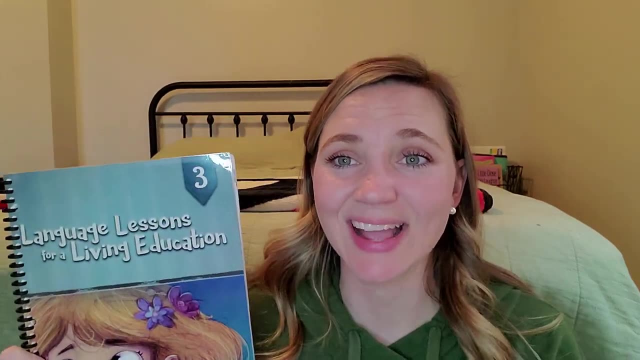 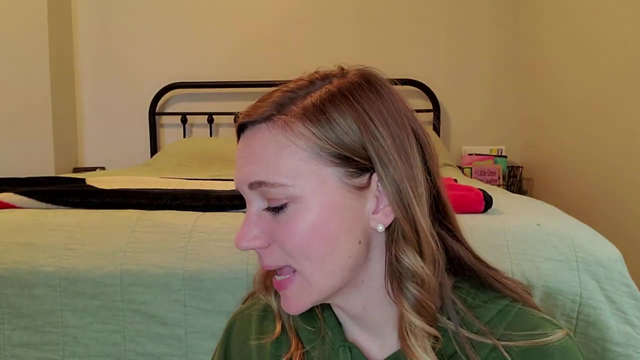 of these. this company is a bad company. It just there was just things that I felt like needed to be in there, that I wanted out of the curriculum I was not getting in this one. So you have the same the same. you get the same schedule. It's laid out. 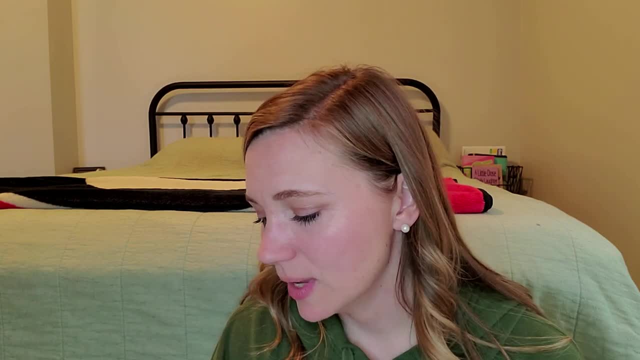 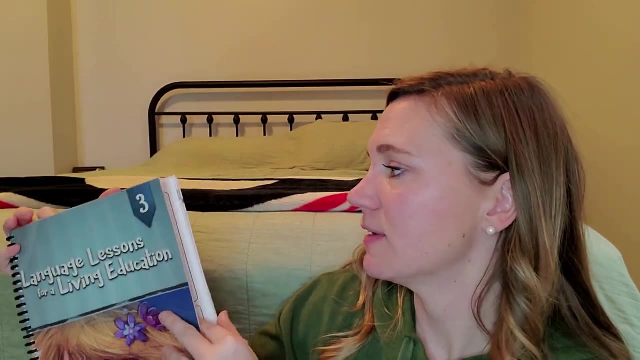 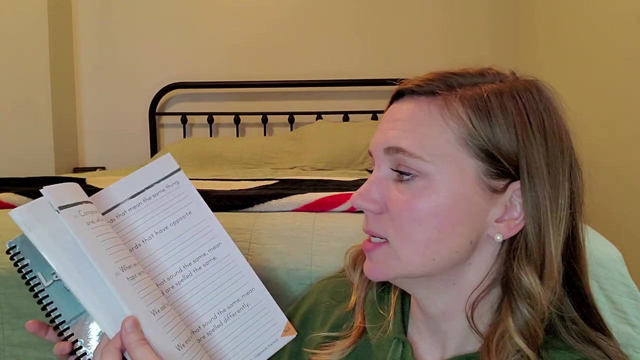 exactly the same as the other one. You get all the copy work, spelling words, review sheets. it gives you games and all of that stuff in the very back for the teacher aid. You have this, the teacher, the answer key. you got the study sheets. 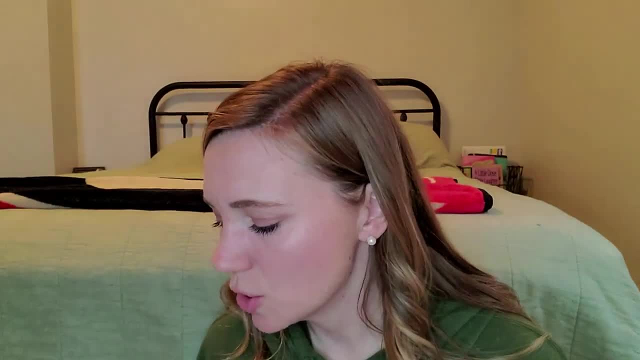 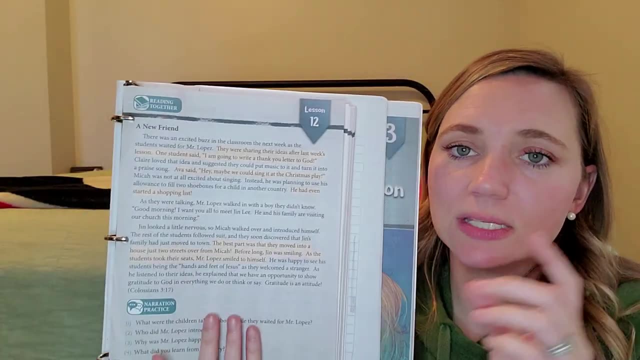 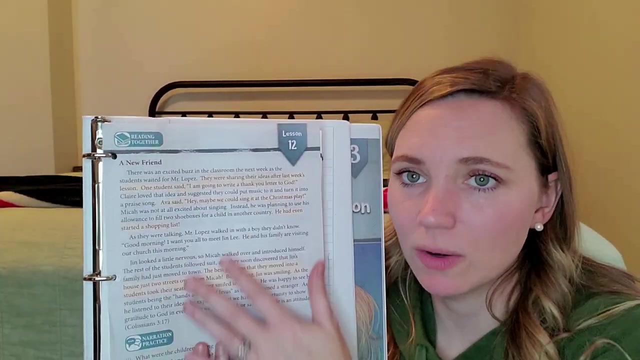 All of that stuff is in the back of that. So how is the same and different from level two? is it set up the same? And the fact that it has the stories, the picture studies and the poems at the beginning of each lesson, or not each lesson, but you know what I mean. Like one week is a story, the next week is 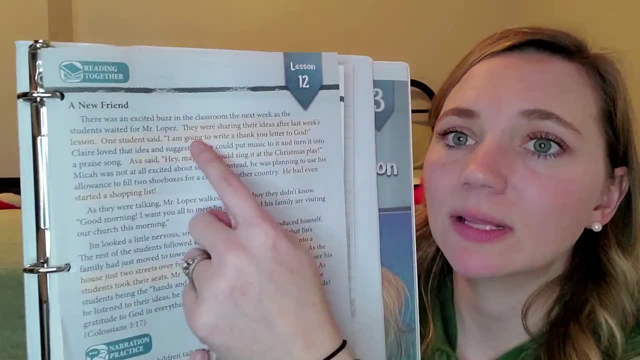 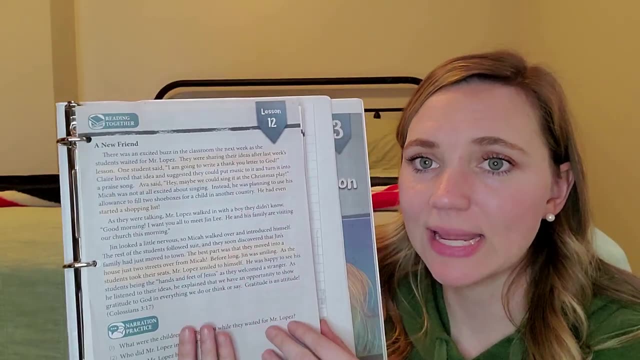 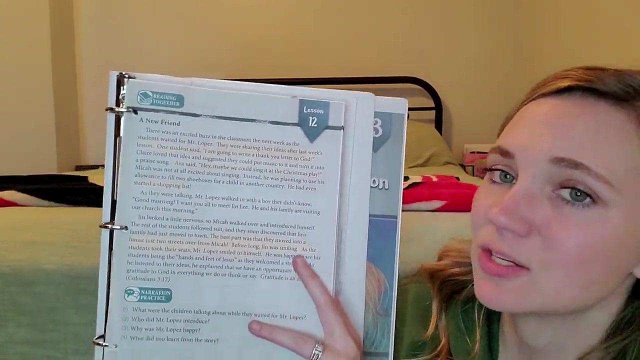 a picture study. the next week is a poem. You have a little bit more highlighted stuff that you need to work through or that your child will read. So there's more reading And again it's a little bit, it's progressively more as you move through the. so like here is lesson 12.. That's what they're reading. 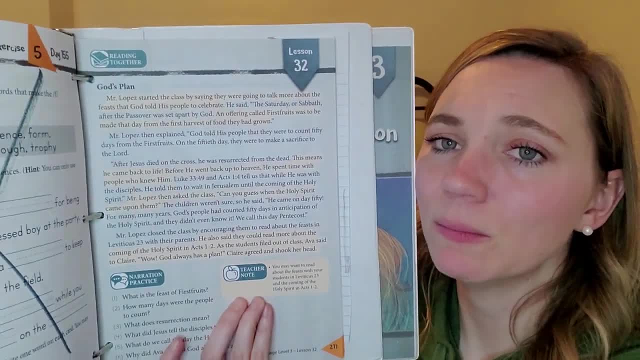 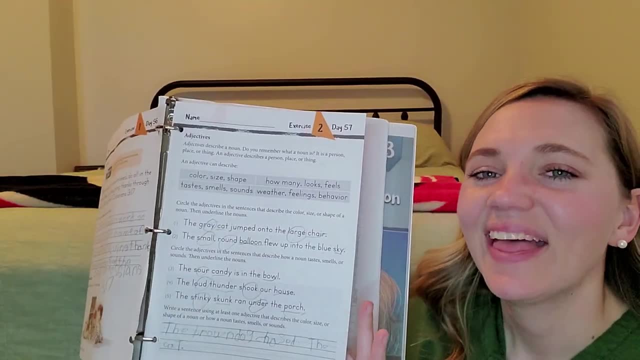 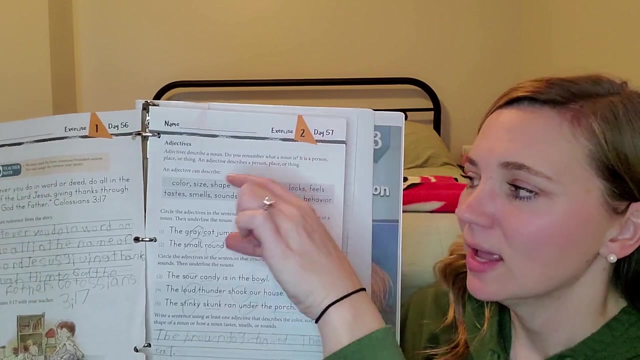 in lesson 12.. Here is lesson 32.. There's a little bit more highlighted there, So there's copy work in here as well. It goes over the grammar stuff And work again the same thing like this would be your teaching And. 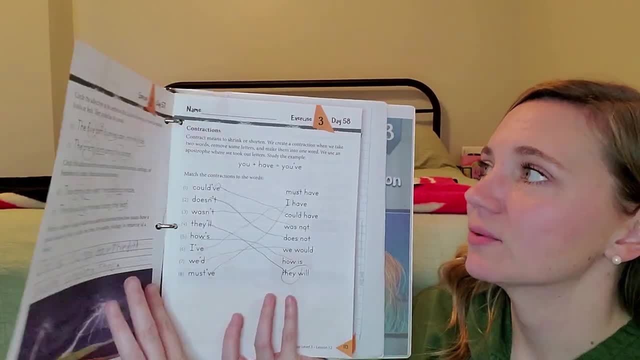 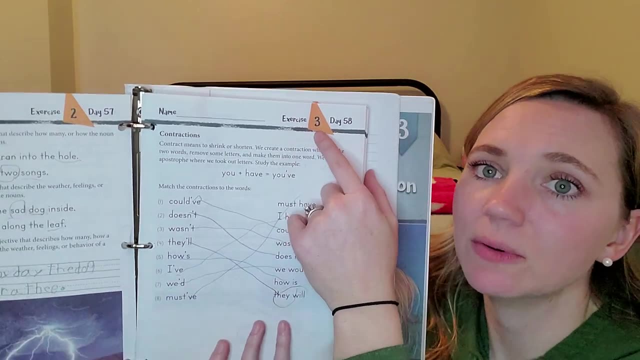 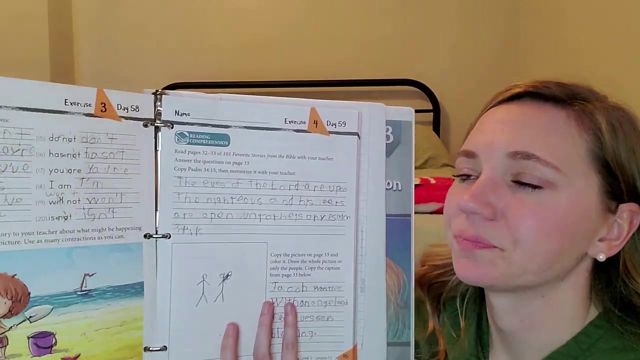 then this is what they would be doing: their worksheet through that. And then exercise two is day two of the week, So that would be like Tuesday, And then exercise three would be Wednesday, And so this is what you're teaching, This is what they're doing. So and again on the back, then on day: 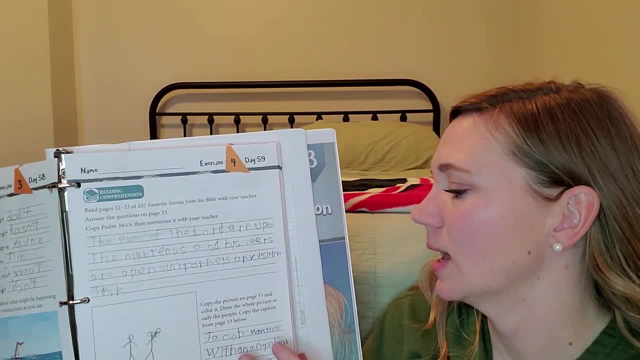 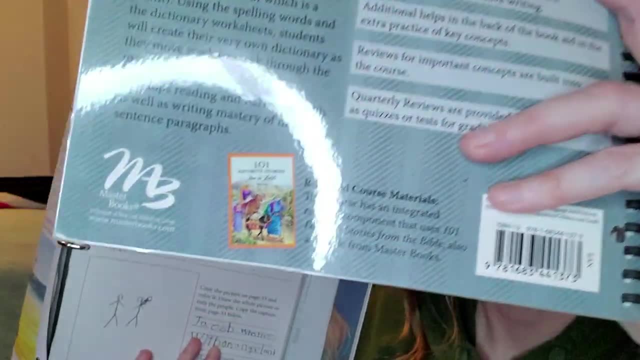 four, you have reading comprehension. So there is a book and I don't have it. Let's see, There it is. I don't have it because I have already sold it. So this, you can see that through my ring light. 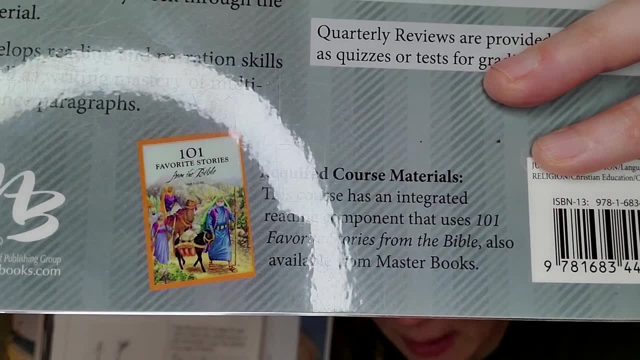 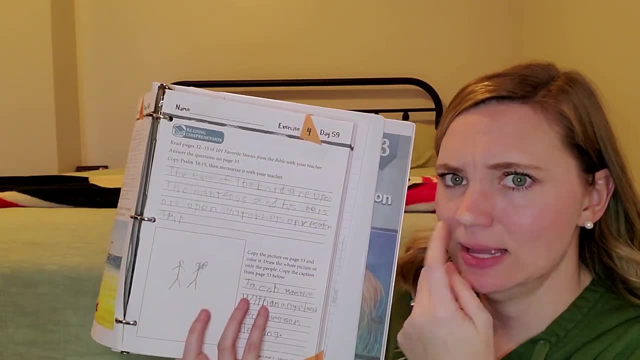 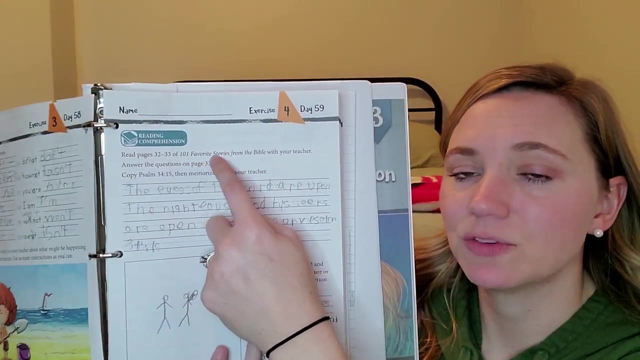 It is 100 favorite stories from the Bible. This is a companion that needs to come with level three and four, I think, and maybe five, But you do have to buy that extra, And so on that day, you will read the pages that it designates for you to read with your 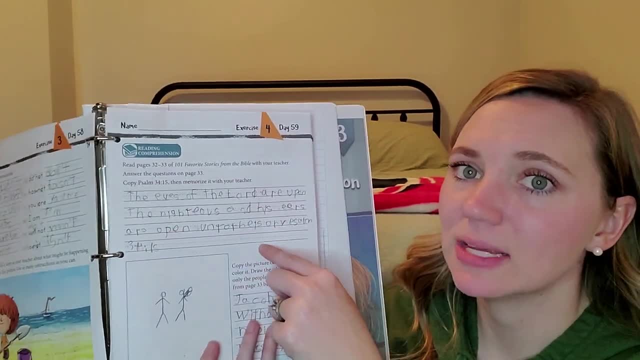 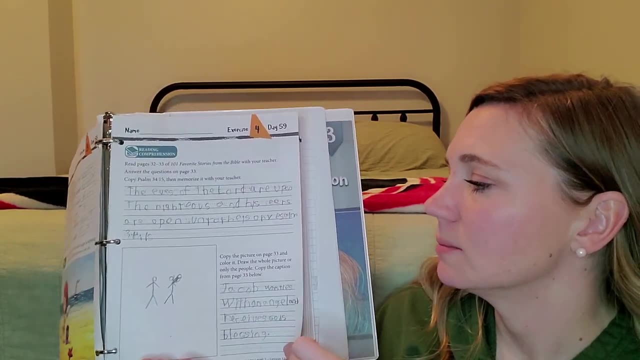 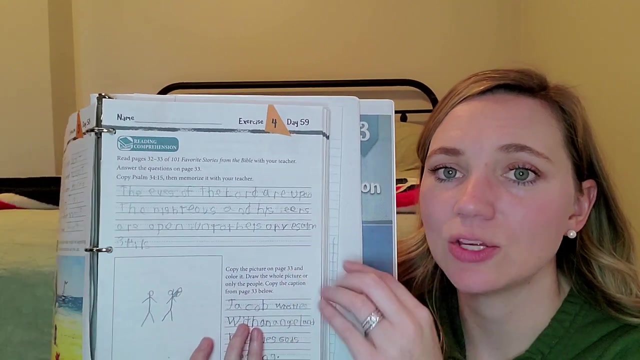 kid. And then they will copy the verse and memorize it with your teacher, And then they will copy the picture that was on that page. And then they will copy the caption. That was day four. Jamison absolutely hated this. When we got to this day, he shut down And so it was like: okay, I can't have you. 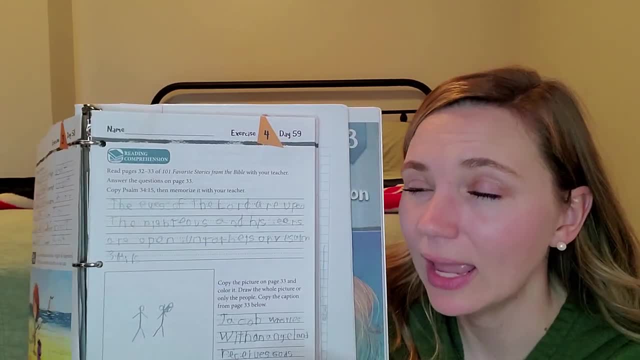 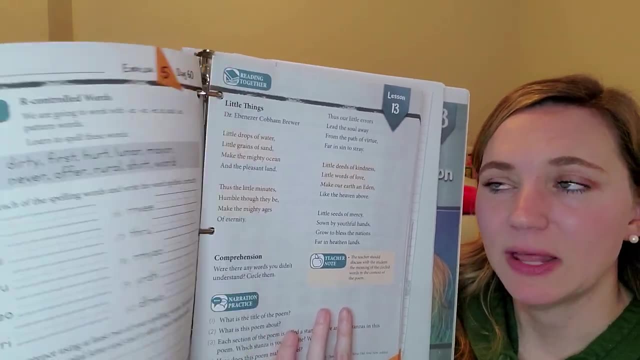 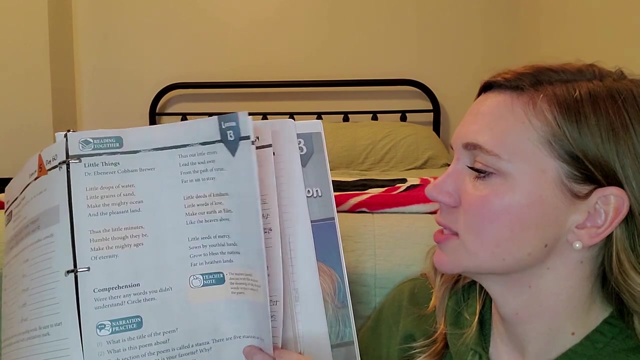 doing that. He just he did not like it. He hated this day of school. And then day five again is spelling. So here is the poem when I was talking about with the poem that went with it, And then I'll show you a picture: study. 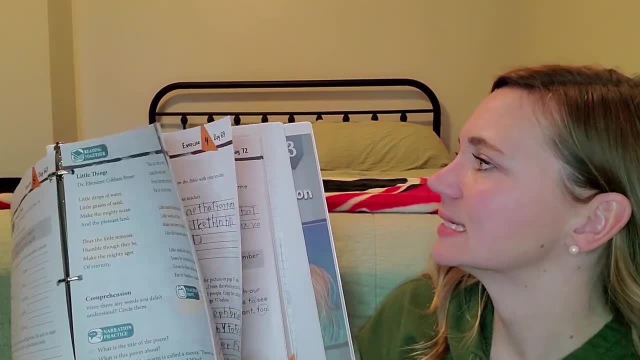 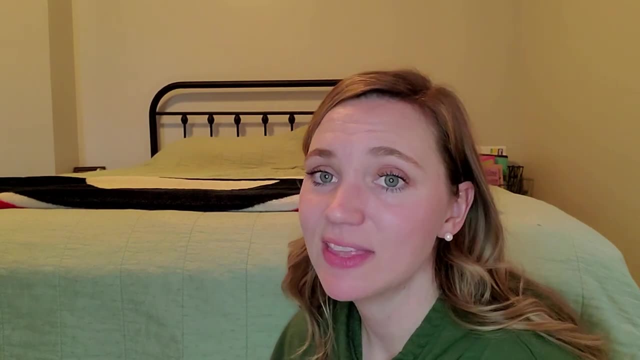 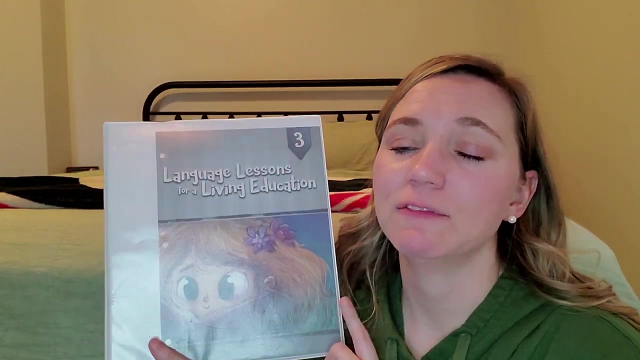 Since I did not show you that, And so here is a picture study, And then you just have questions. to summarize: Not that this curriculum is bad. I think there is a time and a place for it. I think it is very good if you are in a busy season of life And if you just 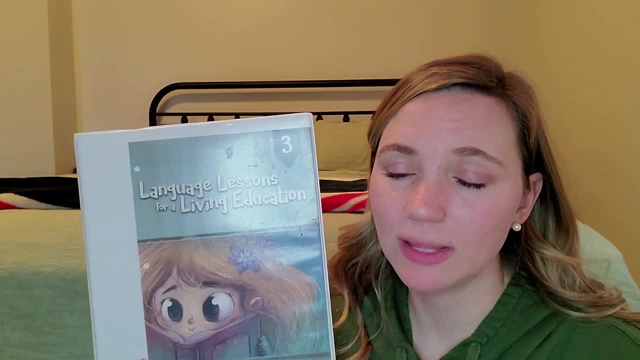 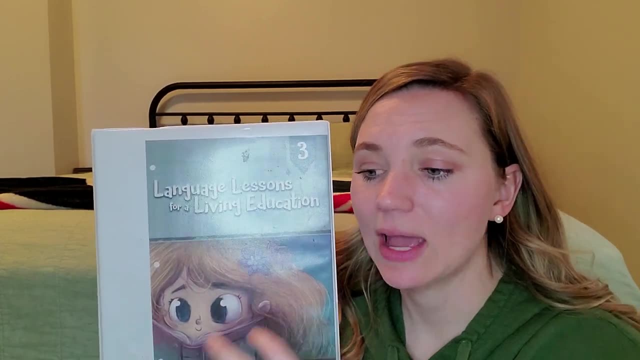 need to open and go. I think this is very good if you have somebody that is struggling- Although I feel like it didn't come back to subjects, didn't come back to concepts- and help you really learn a lot about the Bible. So I think it is very good if you have somebody that is.